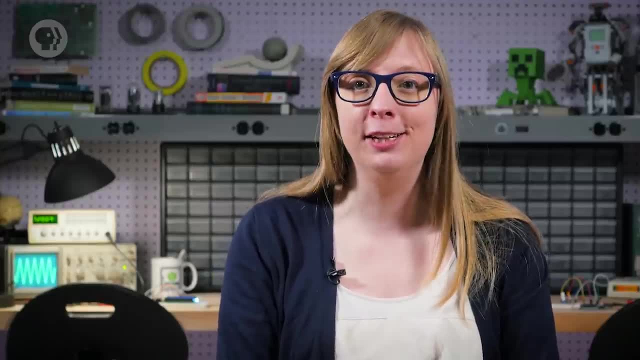 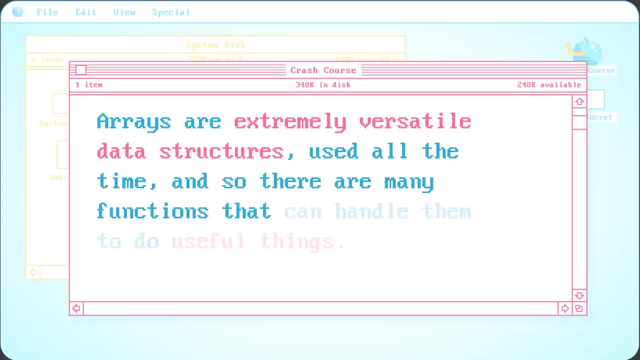 are NOT the same. Remember, the number at index 5 is the sixth number in the array because the first number is at index 0.. Arrays are extremely versatile data structures used all the time, and so there are many functions that can handle them to do useful things. 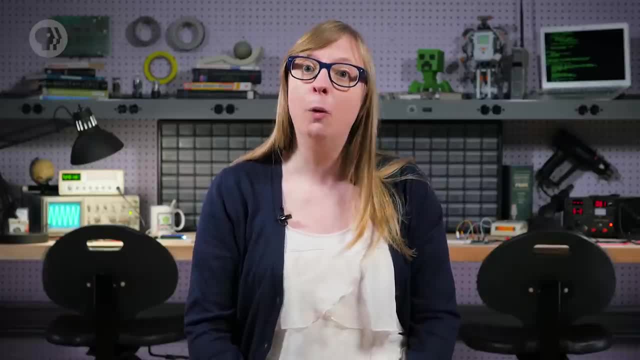 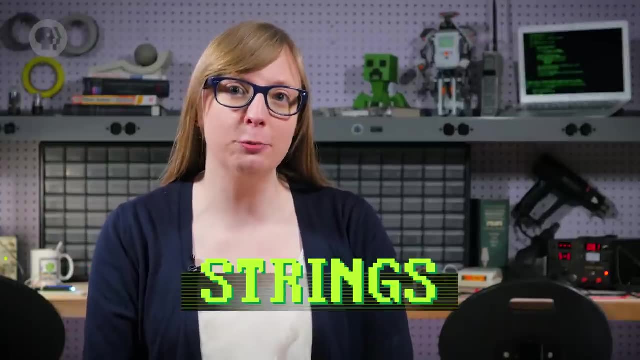 For example, pretty much every programming language comes with a built-in sort function where you just parse in your array and it comes back sorted, So there's no need to write that algorithm from scratch. Very closely related are strings, which are just arrays of characters like letters, numbers. 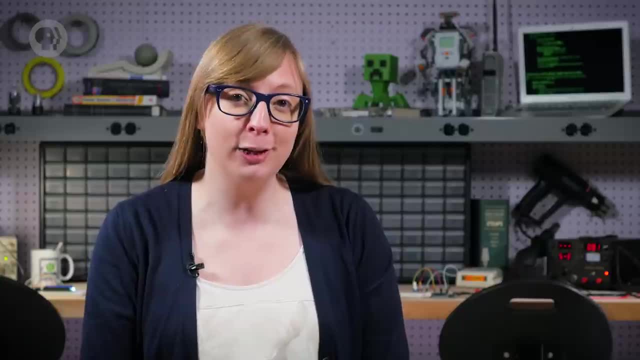 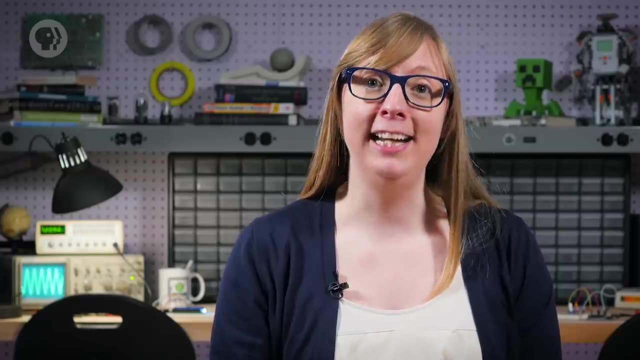 punctuation and other written symbols. We talked about how computers store characters way back in episode 4.. Most often, to save a string into memory, you just put it in quotes like so: Although it doesn't look like an array, it is Behind the scenes the memory looks. 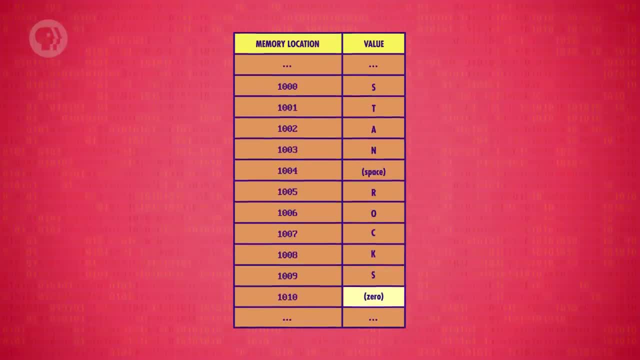 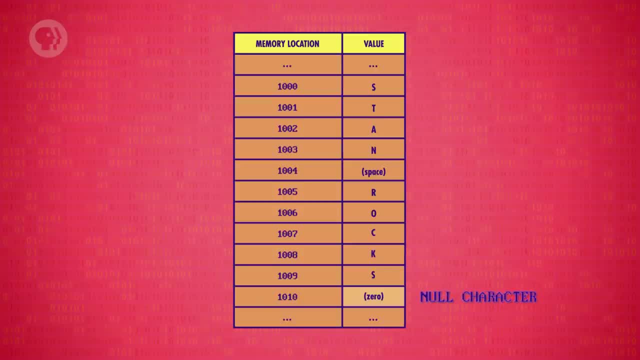 But the binary value zero. This is called the null character and it denotes the end of a string in memory. This is important because if I call a function like printQuote, which writes the string to the screen, it prints out each character in turn, starting at the. 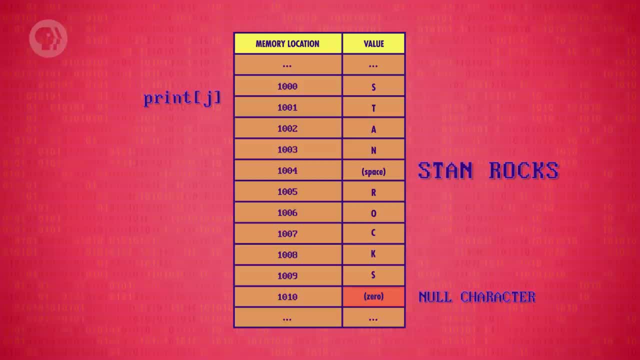 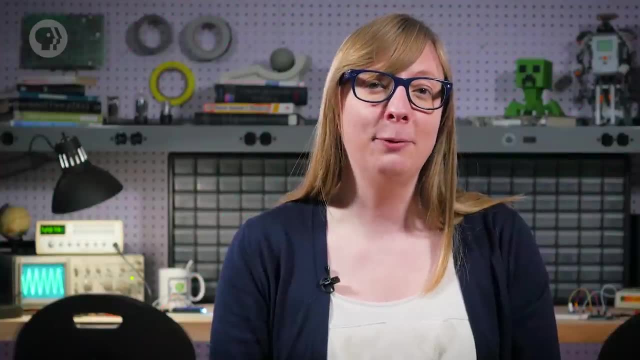 first memory location. But it needs to know when to stop, Otherwise it would print out every single thing in memory as text. The zero tells the string functions when to stop. Because computers work with text so often there are many functions that specifically. 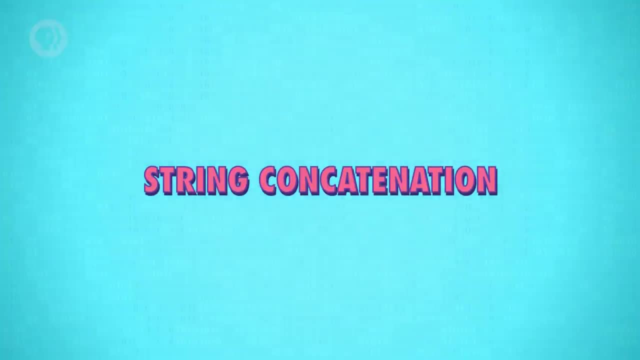 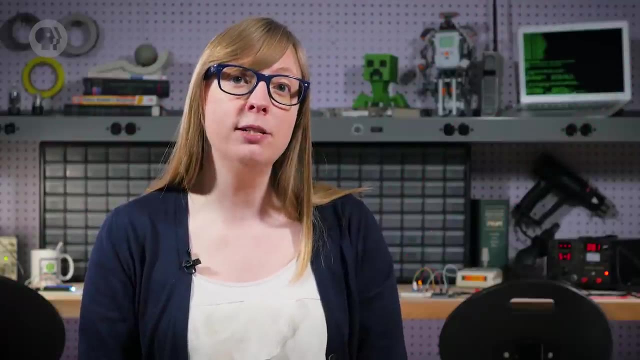 handle strings. For example, many programming languages have a string function, string concatenation function or stringcat, which takes in two strings and copies a second one to the end of the first. We can use arrays for making one-dimensional lists, but sometimes you want to manipulate. 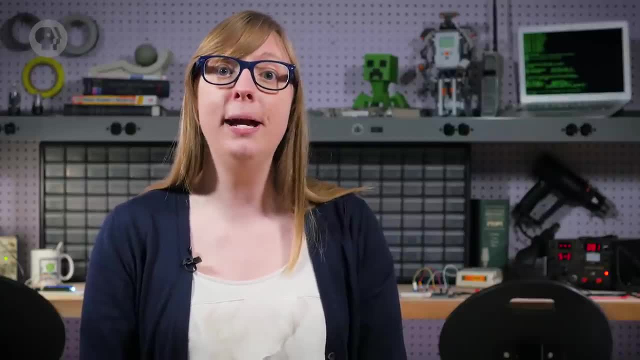 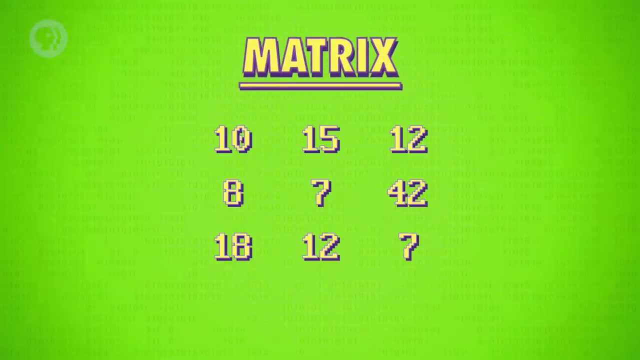 data that is two-dimensional, like a grid of numbers in a spreadsheet or the pixels on your computer screen. For this we need a matrix. You can think of a matrix as an array of arrays. So a 3x3 matrix is really an array of size 3, with each index storing an array of size. 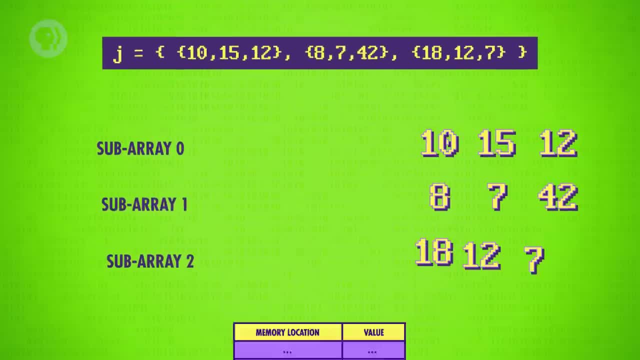 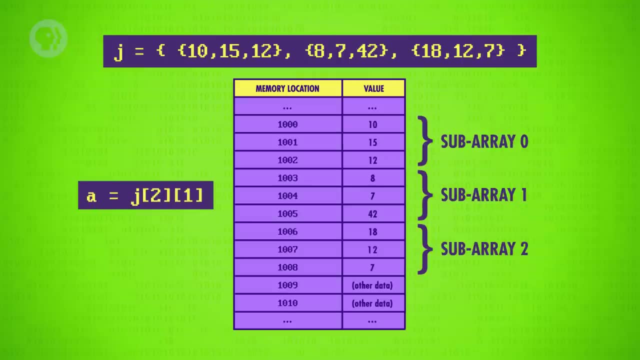 3. We can initialize a matrix like so In memory this is packed together. in order, like this, To access a value, you need to specify two indexes like jindex, then index. This tells the computer you're looking for the item in subarray 2, at position 1.. 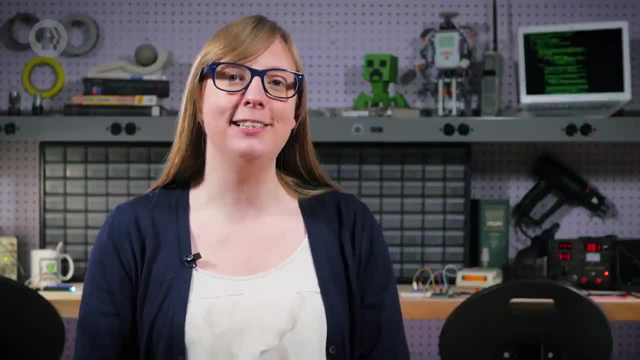 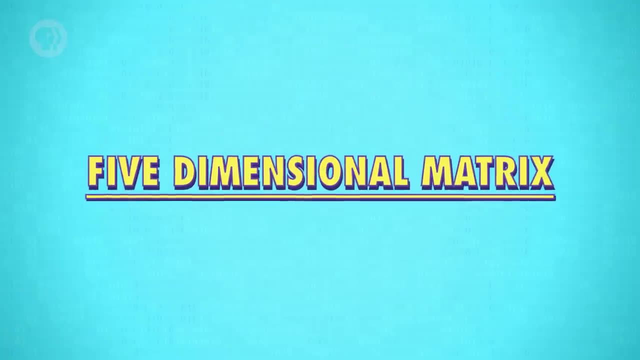 And this would give us the value 12.. The cool thing about matrices is we're not limited to 3x3.. We can make them any size we want, and we can also make them any number of dimensions we want. For example, we can create a 5-dimensional matrix and access it like this: 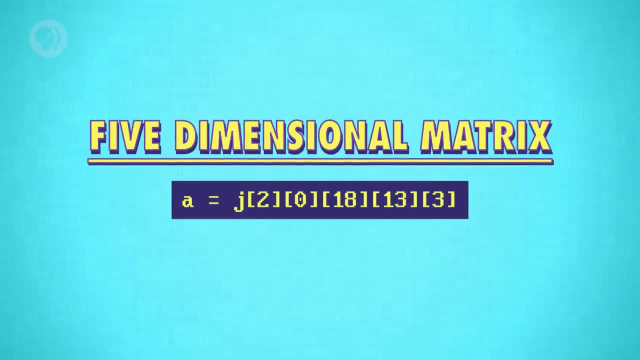 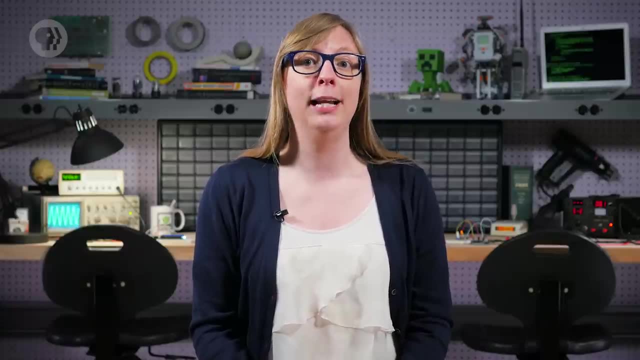 That's right. you now know how to access a 5-dimensional matrix. Tell your friends. So far we've been storing individual numbers or letters into our arrays or matrices, But often it's useful to store a block of related variables together. 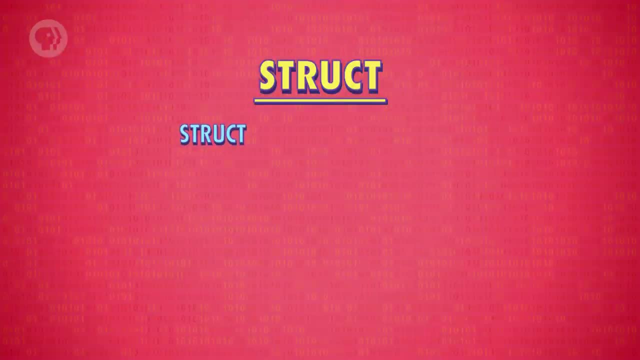 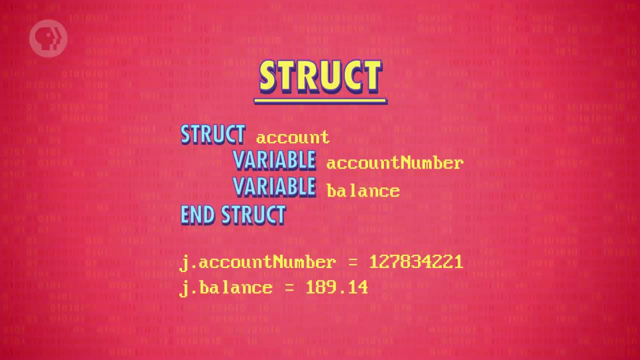 Like you might want to store a bank account number along with its balance. Groups of variables like these can be bundled together into a struct. Now we can create variables that aren't just single numbers, but are compound data structures able to store several pieces of data at once. 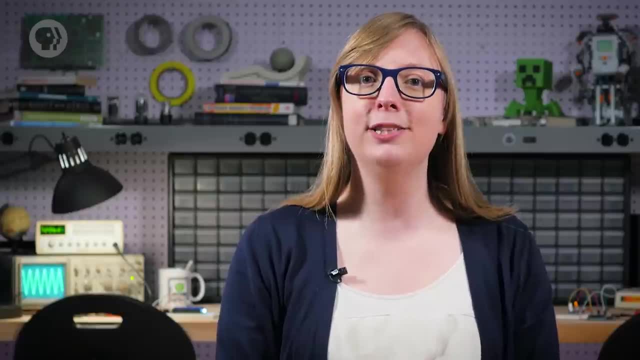 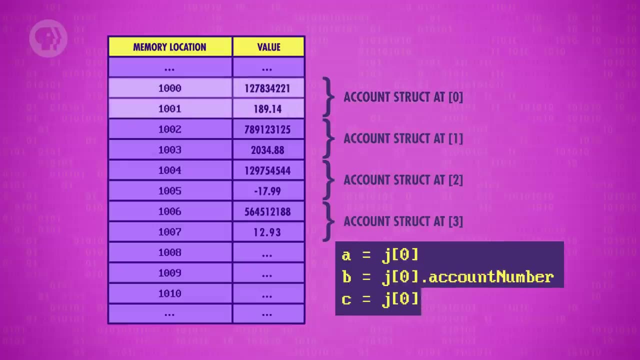 We can even make arrays of structs that we define which are automatically bundled together in memory. If we access, for example, jindex, we get back the whole struct's structure And we can pull the specific account number and balance data we want. 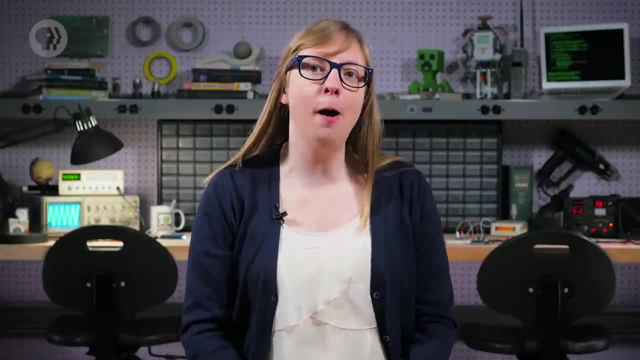 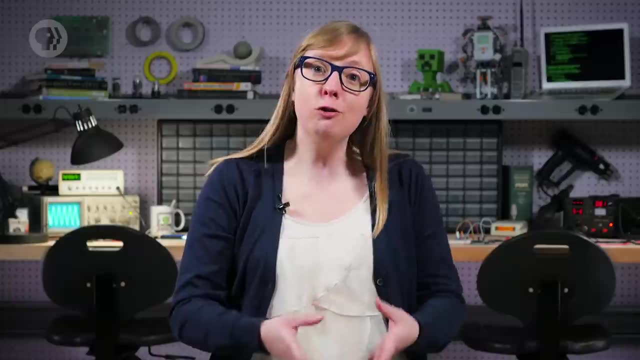 This array of structs, like any other array, gets created at a fixed size that can't be enlarged to add more items. Also, arrays must be stored in order in memory, making it hard to add a new item to the middle. But the struct data structure can be used for building more complicated data structures. 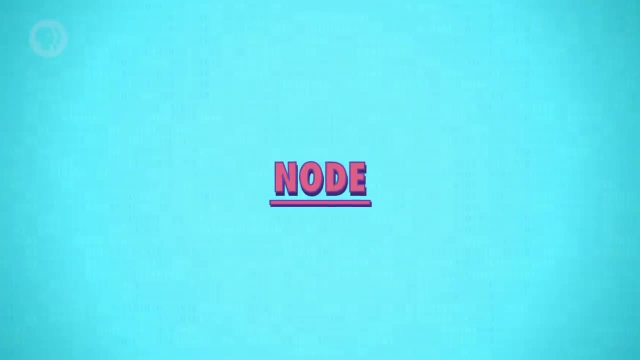 that avoid these restrictions. Let's take a look at this struct. that's called a node. It stores a variable like a number, and also a pointer. A pointer is a special variable that points- hence the name- to a location in memory. 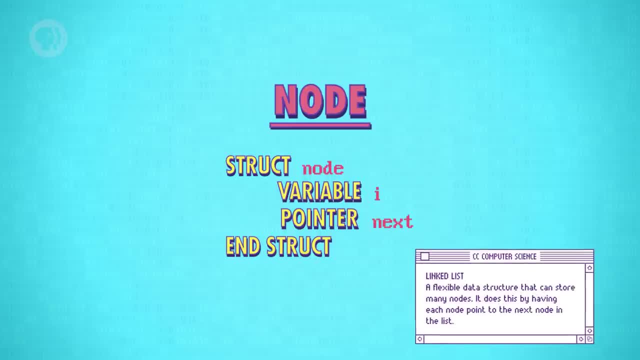 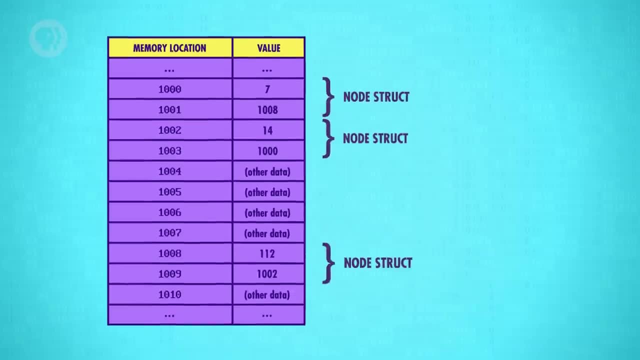 Using this struct, we can create a linked list, which is a flexible data structure that can store many nodes. It does this by having each node point to the next node in the list. Let's imagine we have three node structs saved in memory at locations 1000, 1002, and. 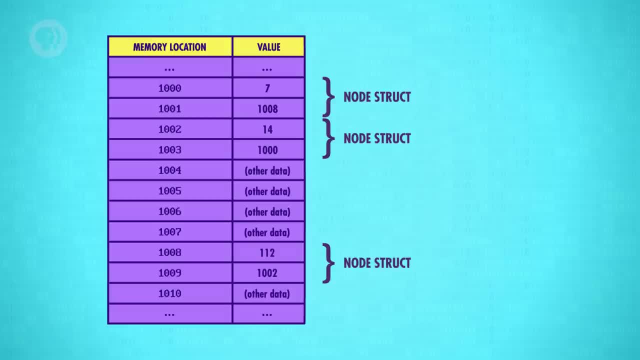 1008.. They might be spaced apart because they were created at different times and other data can sit between them. So you see that the first node contains the value 7, and the location 1008 in its next pointer. This means that the next node in the linked list is located at memory location 1008.. 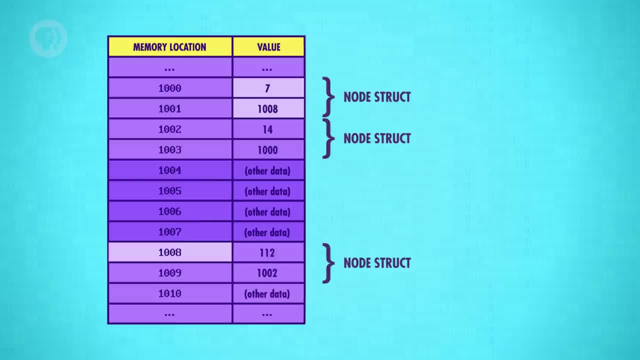 So we can see that the first node contains the value 7, and the location 1008 in its next pointer. Looking down the linked list to the next node, we see it stores the value 112, and points to another node at location 1002.. 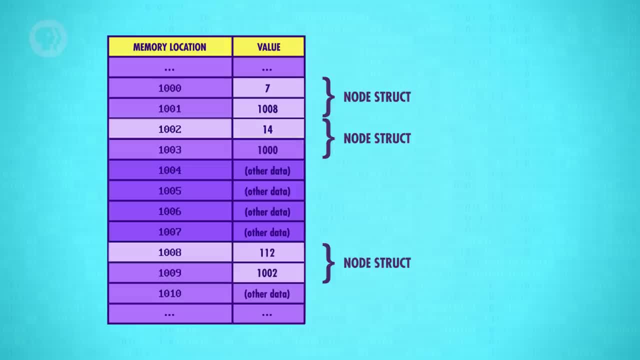 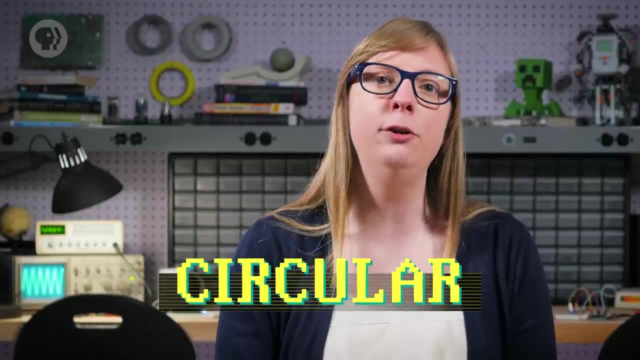 If we follow that, we find a node that contains the value 14, and points back to the first node at location 1000.. So this linked list happened to be circular, but it could also have been terminated by using a next pointer value of 0,, the null value, which would indicate we've reached. 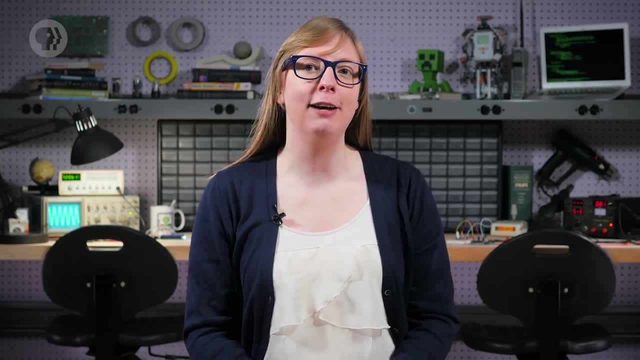 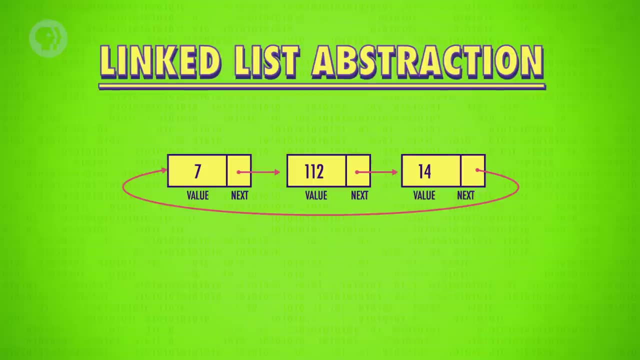 the end of the list. When programmers use linked lists, they rarely look at the memory values stored in the next pointers. Instead, they can use an abstraction of a linked list, A linked list that looks like this, which is much easier to conceptualize: 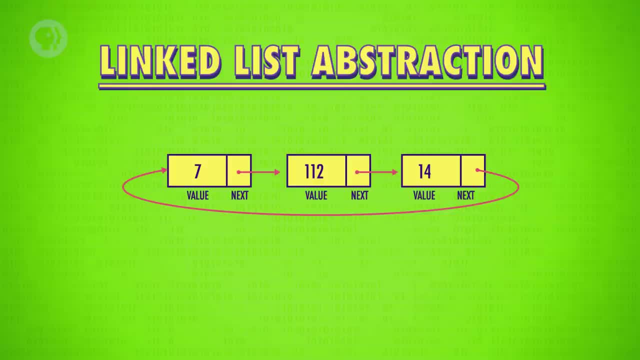 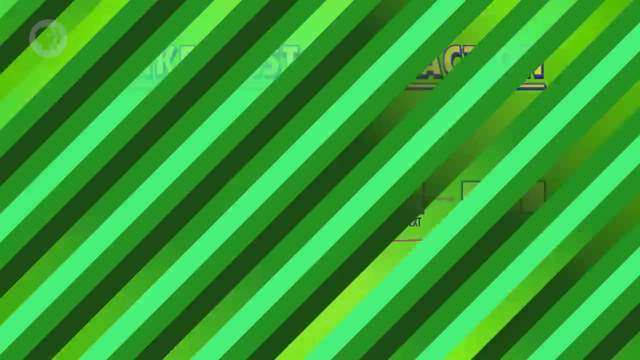 Unlike an array whose size has to be predefined, linked lists can be dynamically extended or shortened. For example, we can allocate a new node in memory and insert it into this list just by changing the next pointers. Linked lists can also easily be reordered, trimmed, split, reversed, and so on, which. 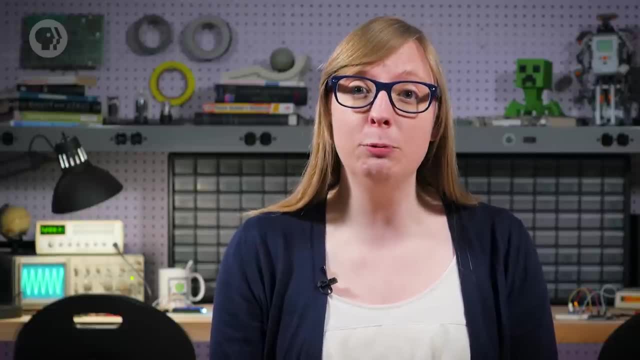 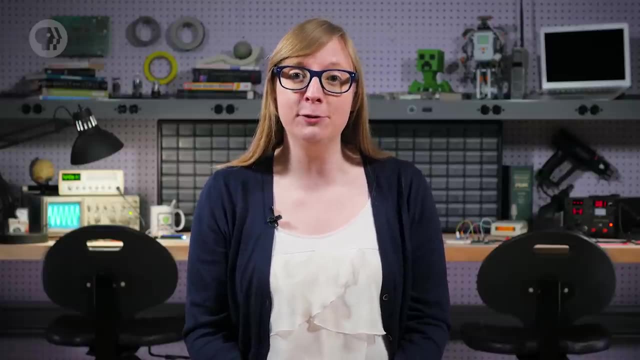 is pretty nifty and pretty useful for algorithms like sorting, which we talked about last week. Owing to this flexibility, many more complex data structures are built on top of linked lists. The most famous in Universal are queues and stacks. A queue like the line at your post office goes in order of arrival. 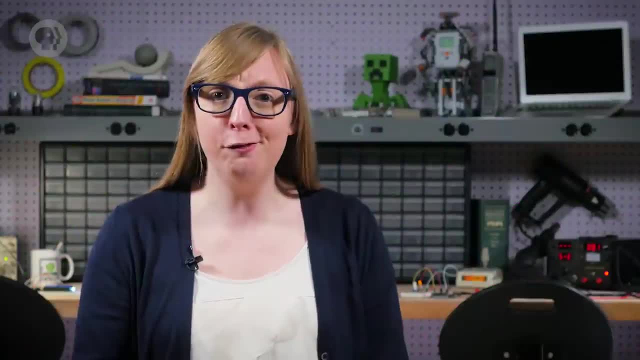 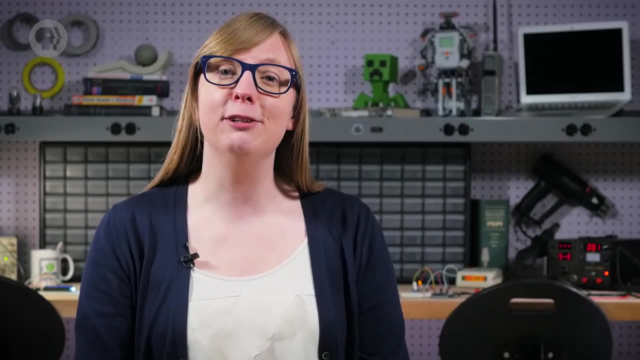 The person who has been waiting the longest gets served first, No matter how frustrating it is that all you want to do is buy stamps and the person in front of you seems to be mailing 23 packages, but regardless, this behavior is called first. 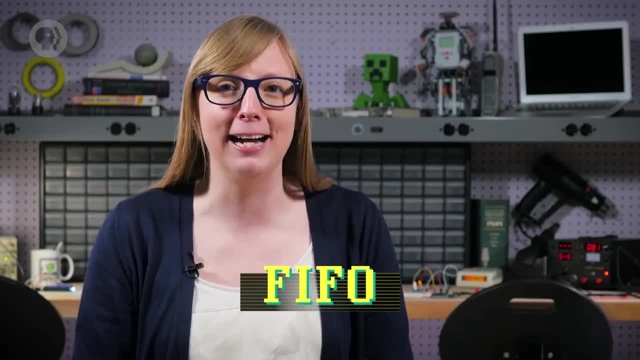 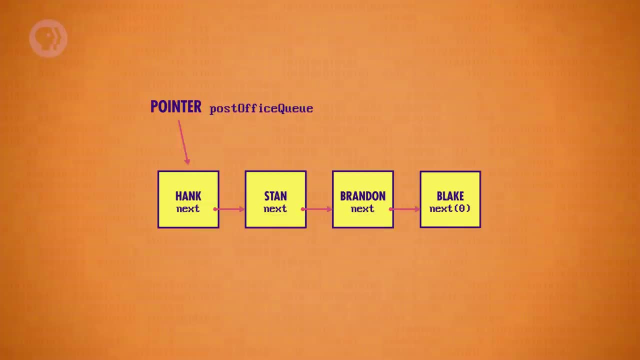 in first out of FIFO. That's the first part, not the 23 packages thing. Imagine we have a pointer named Post Office Queue. that points to the first node in our linked list. Once we've done serving Hank, we can read Hank's next pointer. 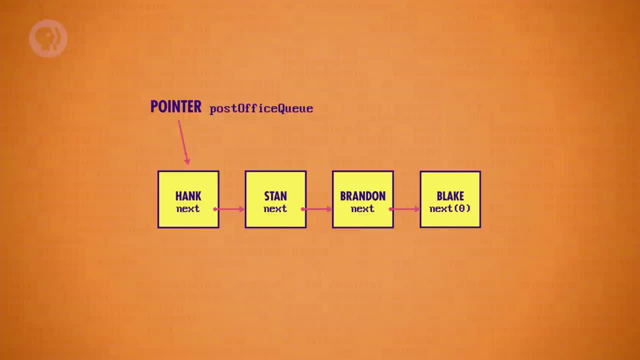 And update everything. We can also update our Post Office Queue pointer to the next person in the line. We've successfully dequeued Hank. He's gone, done, finished. If we want to enqueue someone, that is, add them to the line we have to traverse down. 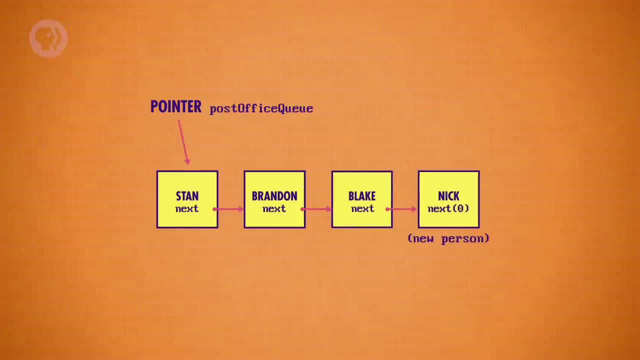 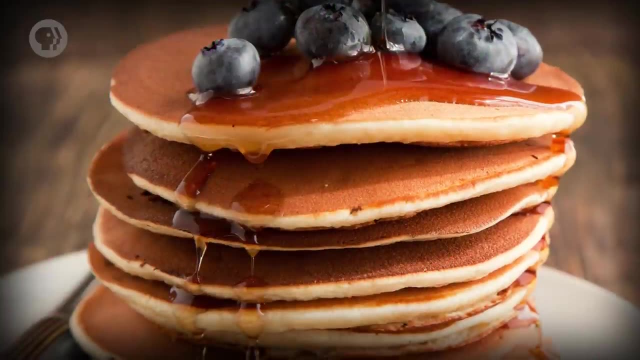 the linked list until we hit the end and then change that next pointer to point to the new person. With just a small change, we can use linked lists as stacks, which are LIFO – last in, first out. You can think of this like a stack of pancakes. 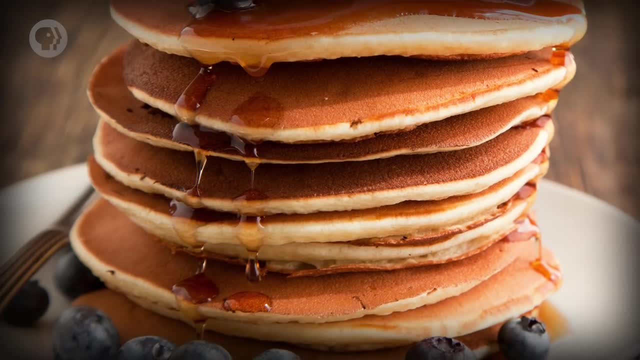 As you make them, you add them to the top of the stack, and when you want to eat one, you take them from the top of the stack. Delicious. Instead of enqueuing and dequeuing, data is pushed onto the stack and popped from. 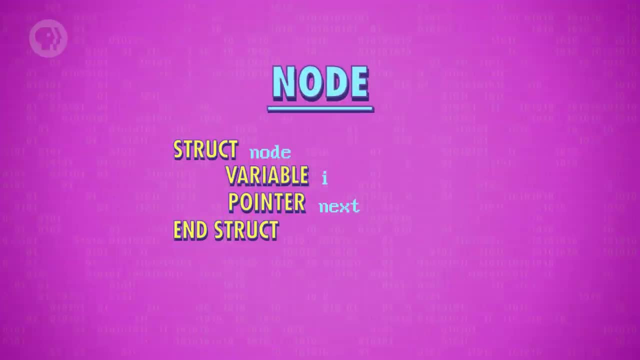 the stack. Yep, those are the official terms. If we update our node struct to contain not just one but two pointers, we can build trees – another data structure that's used in many algorithms. Again, programmers rarely look at the values of these pointers and instead conceptualize. 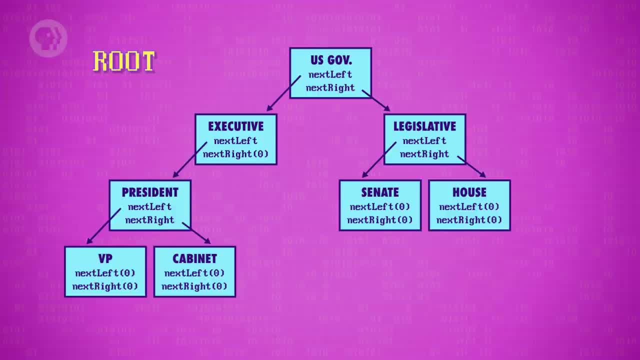 trees like this, The topmost node is called the root and any nodes that hang from other nodes are called children nodes. As you might expect, nodes above children are called parent nodes. Does this example imply that children are parent nodes? Does it imply that Thomas Jefferson is the parent of Aaron Burr? 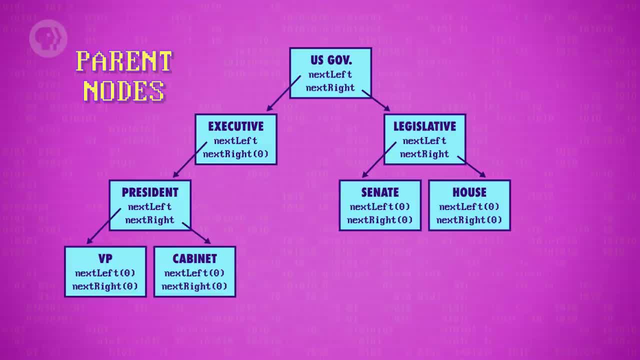 I'll leave that to your fanfiction to decide. And finally, any nodes that have no children, where the tree ends are called leaf nodes. In our example, nodes can have up to two children and for that reason, this particular data.